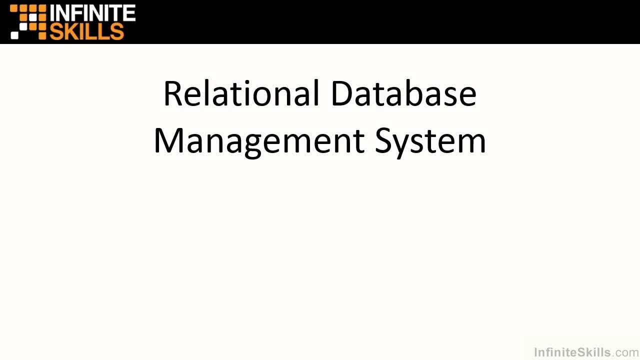 Welcome to SQL S-Q-L Standard Query Language. It's the language for querying databases. Before we actually get into the nuts and bolts of the actual language and all its capabilities, we need to do just a little bit of background cover on databases themselves and, more importantly, on relational databases. 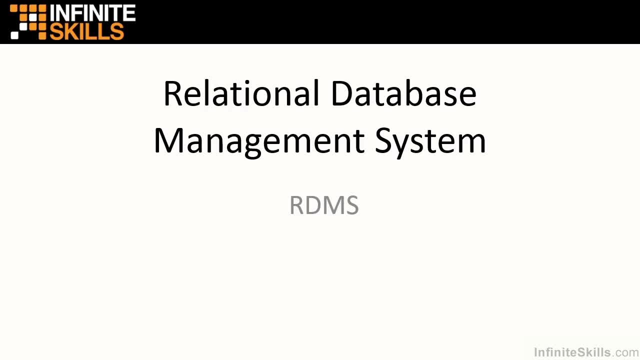 So we need to look at Relational Database Management Systems, or RDMS- much shorter abbreviation. So what is a Relational Database Management System? Well, basically it's a database that has a number of relationships, So it's made up of more than one table, It's not a single table. 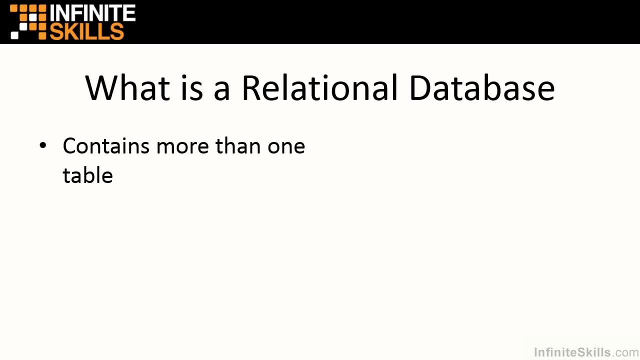 As soon as you have two tables, we are into a relational database, therefore a Relational Database Management System. Between those multiple tables there must be relationships, So there must be a relationship between any given two tables. Now that doesn't mean that there must be millions of relationships between every table in your database. 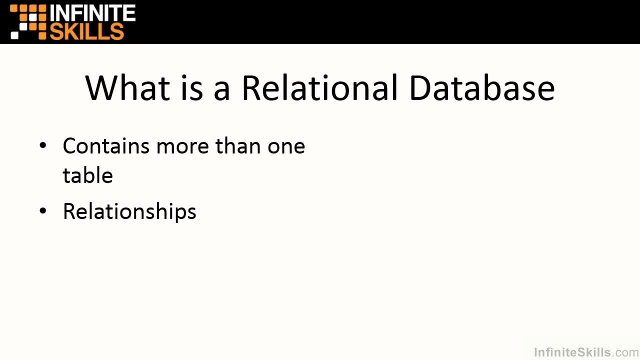 but certainly between one table and another there must be relationships, And then between that table and another, so that you can then effectively link data from table one to table three. You will find that your tables are broken down to parent tables and child tables. 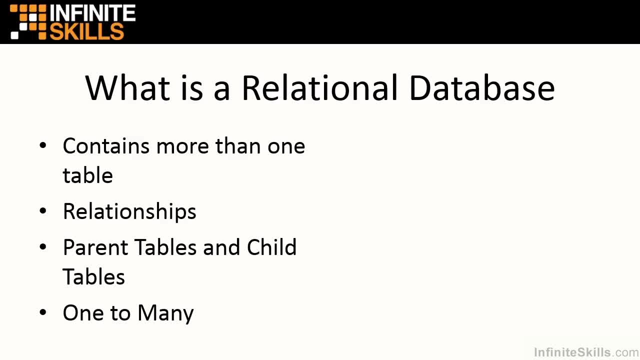 And there exists a one-to-many relationship between each parent table and each child table. The reason that they're given the name of parent and child? because it makes logical sense: You have one parent but potentially many children, hence the little graphic. 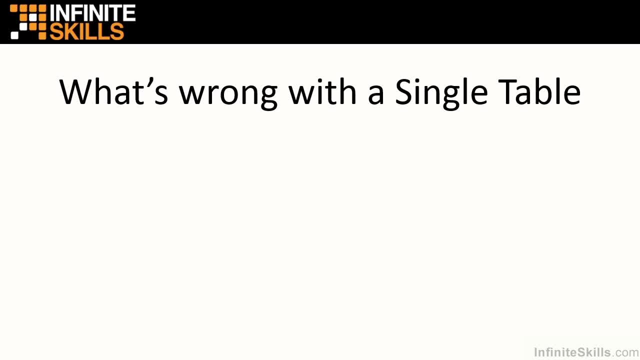 What's wrong with having a single table? Why can't we just have one big table, a bit like Excel or any spreadsheet package, Where you can just create a nice big table and start entering all your data and keep it like that? Well, there are a couple of issues with such large, single tables. 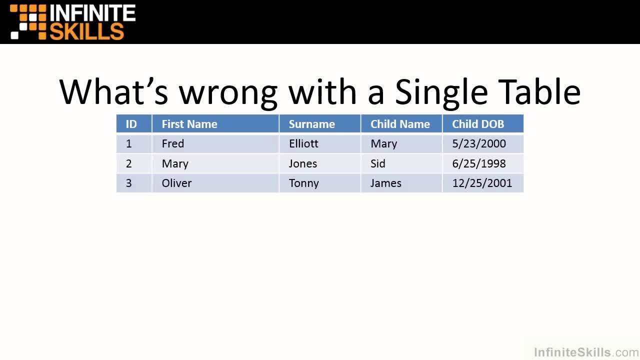 First example of a problem with large single tables comes when you start to have extra data that needs adding in. So if we take a small table here which is our friends, their first name, their surname, their child's name and their child's date of birth, 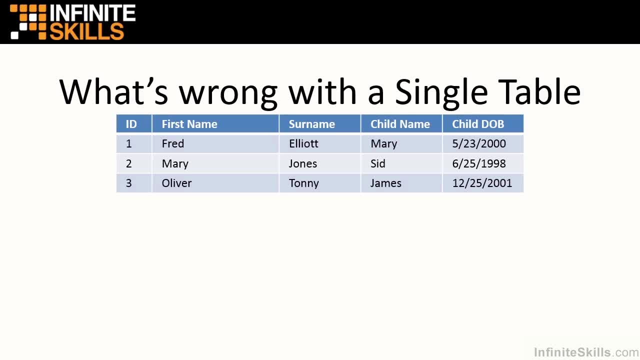 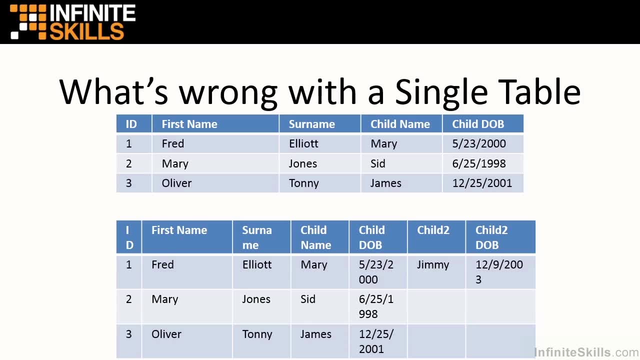 Unfortunately, as soon as one of my friends has a second child, the table needs to be restructured and we need to add in a second table. We need to add in a column for that second child and a second column for that child's date of birth. 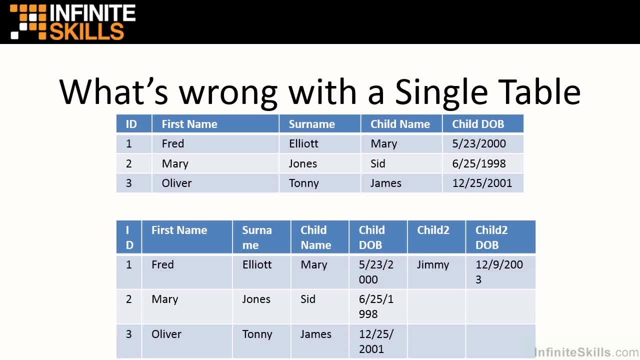 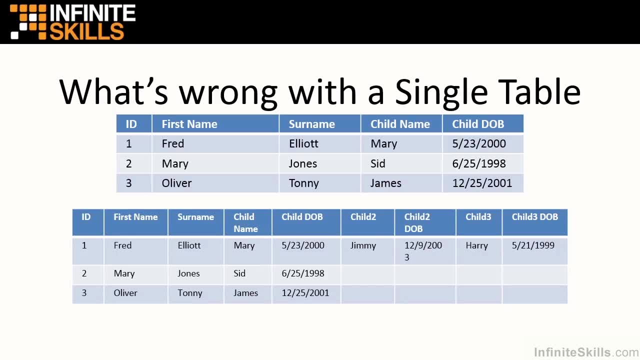 So that's two more columns added to the table. We can see here that Fred Elliott has a second child called Jimmy, but my other two friends, Mary and Oliver, they don't have a second child. We then have a problem when Fred goes and has a third child. another two columns need to be added for child three's name and child three's date of birth. 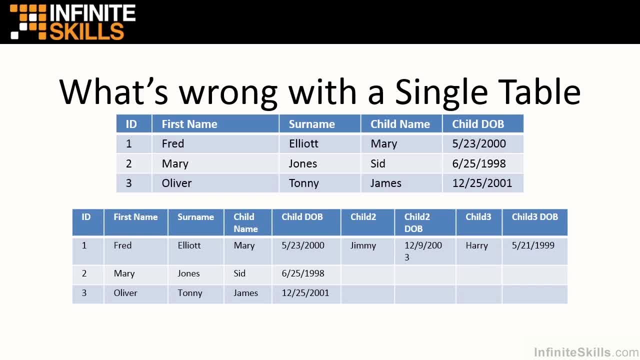 But still again, Mary and Oliver don't have child three, So we've got these empty cells, empty fields, empty boxes. whatever terminology you'd like to use, they are empty. They're effectively not being used. Now, hopefully you can see, this becomes even more of an issue. if someone has four children, five children, six children, your single flat table becomes much, much larger. 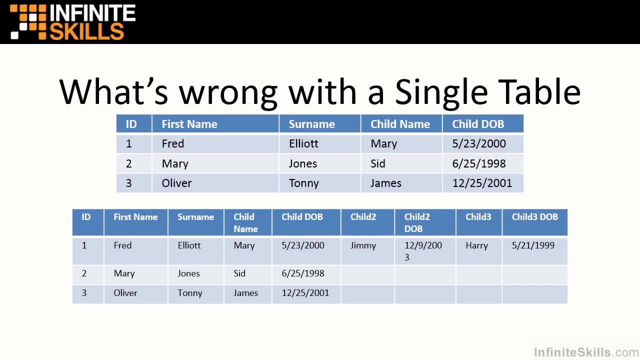 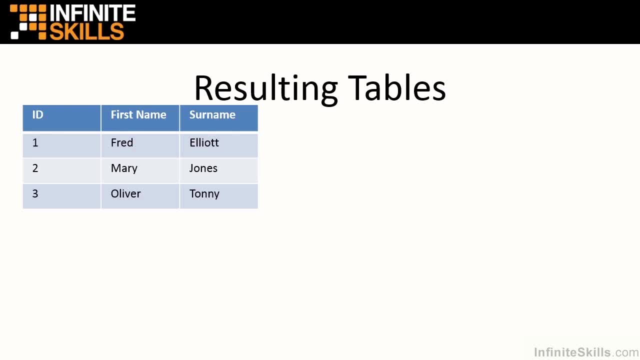 So the plan instead is not to put those children at all in the table with the parents, but to put them in their own table. How this will look is we'll have a single table, no children in here at all, just the first name and the surname of each of my friends. 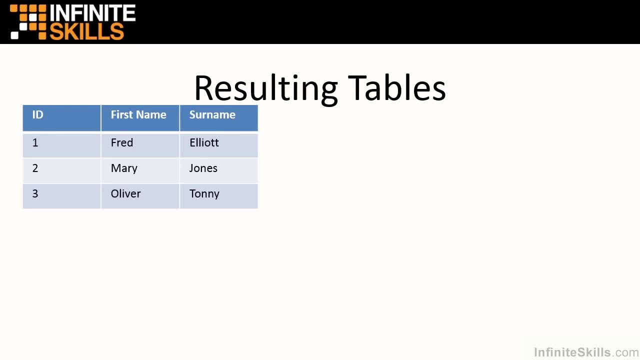 They are given a unique ID. that unique ID is referred to as the primary key. You'll see shortly why We need them to have a unique ID. We then create a second table which contains all the children. So each child is a new record, a new row in our children's table. 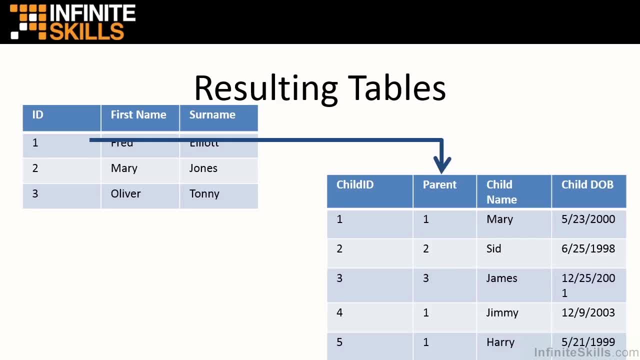 And then we link through to the parents table, a friend's table, using the ID of the friend linked through to the field that we've called parent. So the ID one goes to ID one and we can see that ID one parent has Mary, Jimmy and Harry. 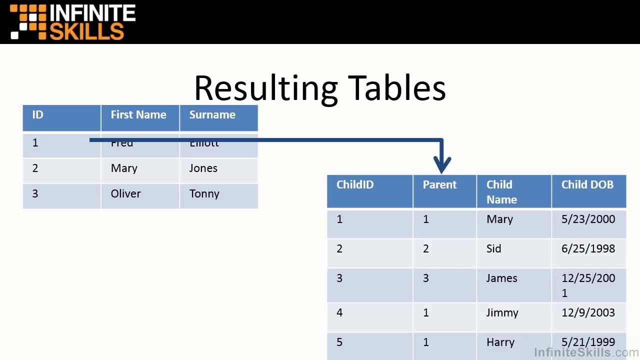 To find out who parent one is, we go back to the parent table and say, oh, one's friend. And then we go back to the parent table and say, oh, one's friend is Fred Elliot. So rather than linking through to the name Fred Elliot, which could repeat, I could have two Fred Elliot's- we link through directly to the primary key, because that's unique. 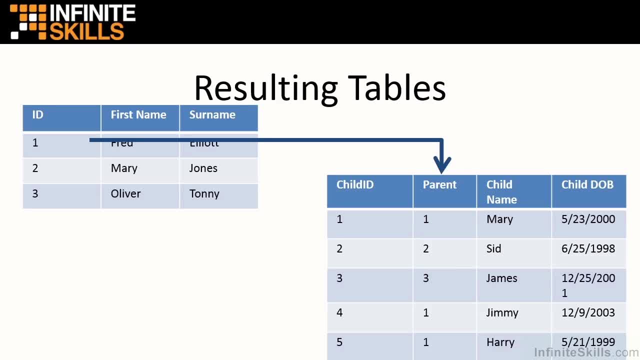 Advantage here is anybody who doesn't have any second or third or fourth or fifth or sixth children, or even any children, just doesn't have an entry in the children's table. So there's no empty rows and there's no restructuring. Fred could now go ahead and have 10,, 15,, 20 children. 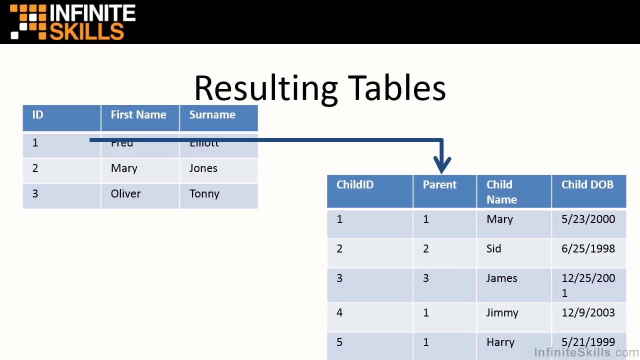 There will be no restructuring of any of the table structures. We would just simply add another row into the children's table. So that's effectively the main reason you'd want to have multiple tables. But there is another reason that's really very helpful to have multiple tables for. 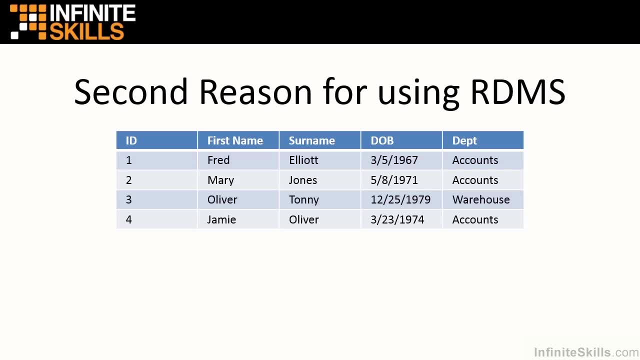 And that's, if you have repeating values, quite common, repeating values in a particular field. You have here, for example, we've got our friends again and we've also put their date of birth and their department. Now, three of my friends work in the same department. 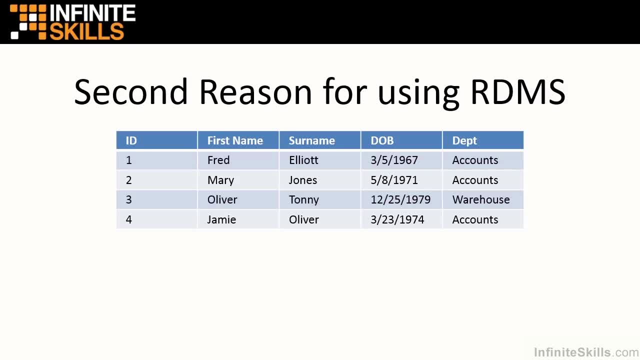 So there's repetition in that column. That's not a problem if there's four entries, but if there's 4,000, 40,000,, 400,000, that means the word accounts. It's repeated numerous times, increasing the chance of it being spelt wrong, increasing the data space required to store it. 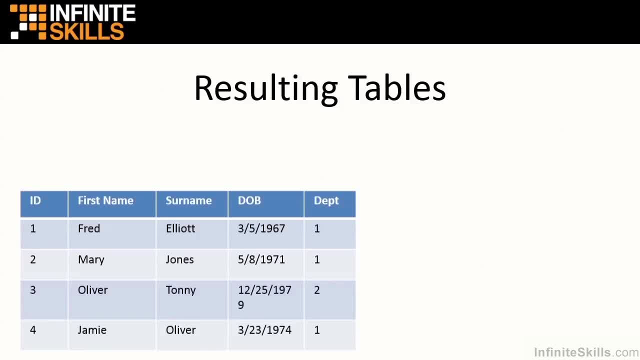 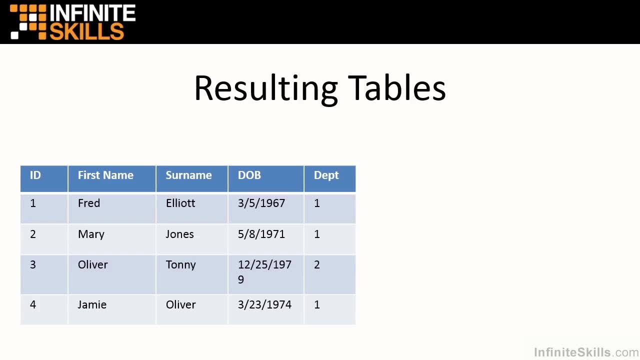 So instead what we do is we have multiple tables- again Friends table, but you'll notice that the departments are now all numbers And Fred, Mary and Jamie work for department number one and Oliver works in department number two. What we've done is removed the text values, placed them in their own table over here and given them a unique ID. 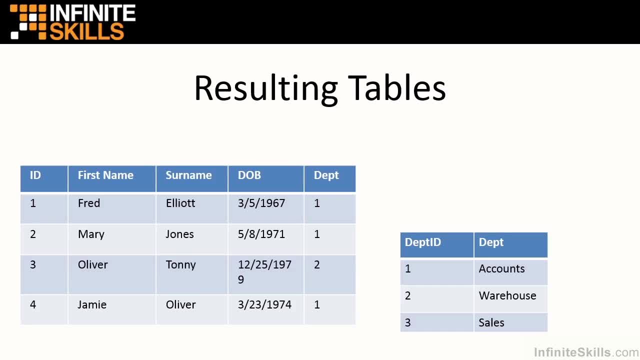 So again it has a primary key. So accounts are department one warehouse, department two sales department, And we link the department ID to the department in our friends table. That way we can see. okay, Oliver works for department two. I'm not really sure what department two is. 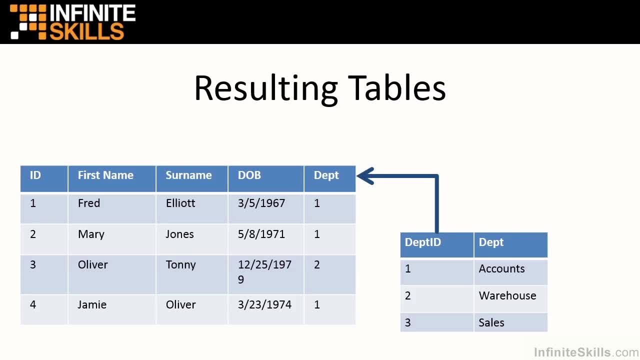 We follow the two through the join and find out the department two is the warehouse department. By doing it this way, the names of each department only appear once in the whole database and that's in the department table. Everywhere else we need to know what department anybody's in or the work's going to. we use the department ID. 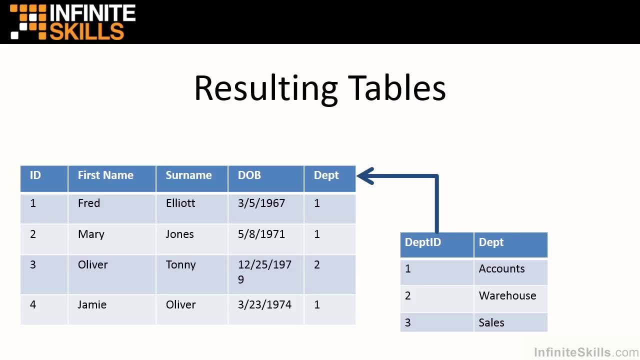 And we can pull out the label as and when required, Because the numbers work much faster in any database system than a string of text. So we've saved the repetition, which will reduce data entry issues, and it will also increase extraction of the data. 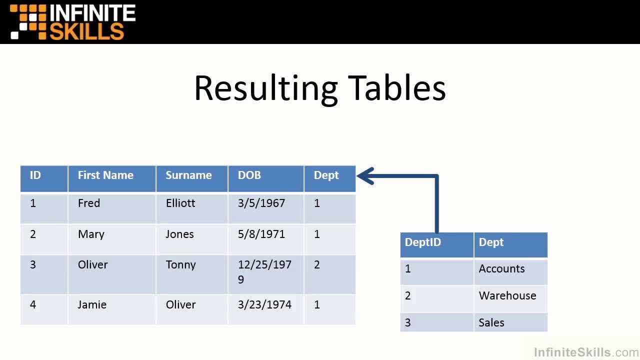 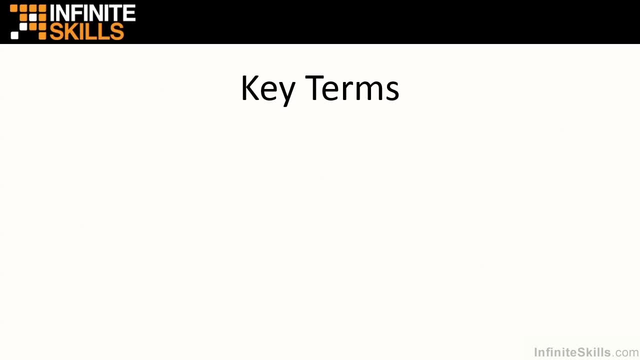 Because we're using numeric values to make that link. So that's relational databases just as a background really to why and wherefore we're going to use standard query language. So the key terms that we've covered are database, which is a single entity of data, but that single entity can contain multiple tables. 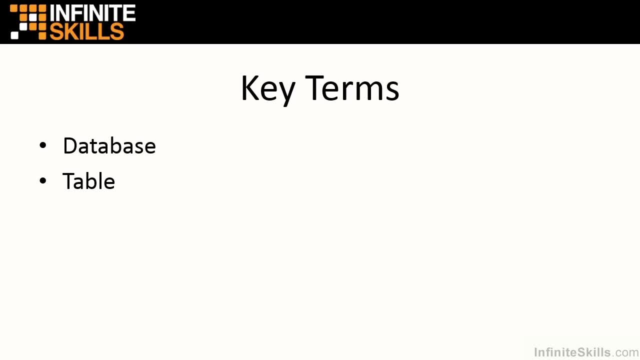 So the key terms that we've covered are database, which is a single entity of data, but that single entity can contain multiple tables, So we have a table. Tables contain data broken out into fields or columns, depending on what you want to call a column of information. 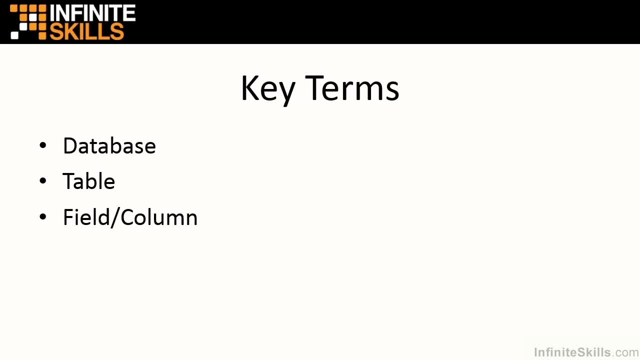 Each column should be a single type of data, So it should be, for example, the first name or the last name or the date of birth. You shouldn't have mixed columns of data, otherwise it becomes very hard to then extract the information that you want.